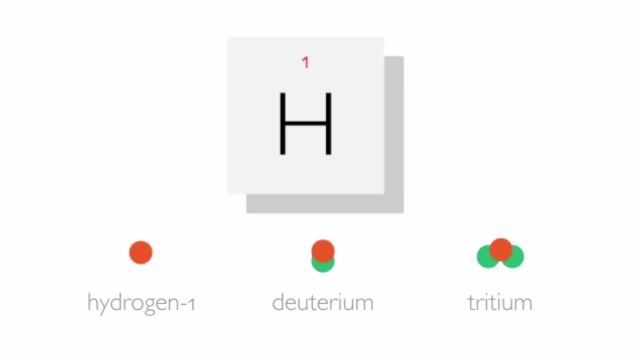 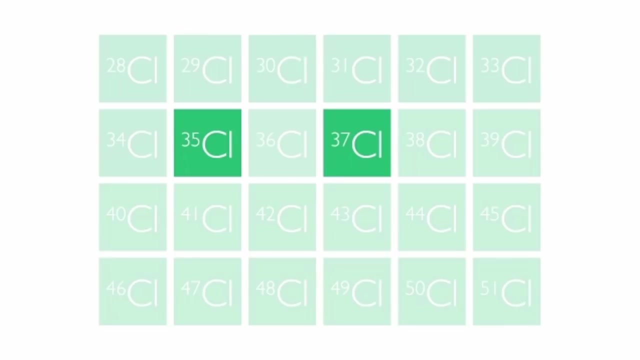 This means that the element is unchanged, and that's the important point. It is still hydrogen and will react chemically in exactly the same way. There is often more than one stable isotope of an element. In fact, much of the world around us is made up of stable isotopes. However, sometimes there aren't enough neutrons in 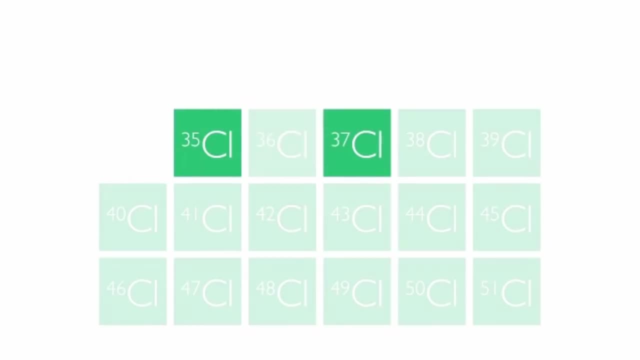 a nucleus. This means that there may be too many to be stable. An analogy is a person carrying boxes. If you try to carry too many boxes, you will end up dropping some, And if you continue, you will keep dropping boxes until you reach. 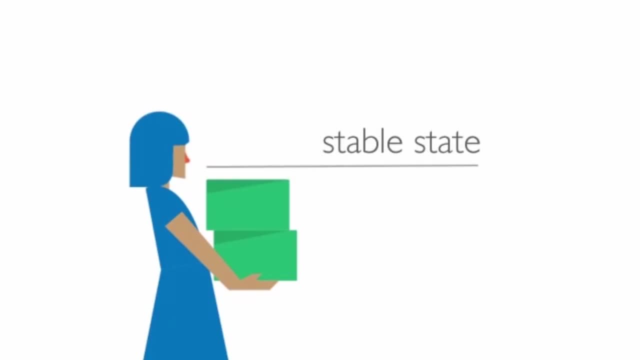 a manageable amount. This is your stable state And nuclei behave in a similar way and they will try to stabilise themselves. If there are too many protons or too many neutrons, the nucleus can spontaneously rearrange itself and throw out particles in the process. 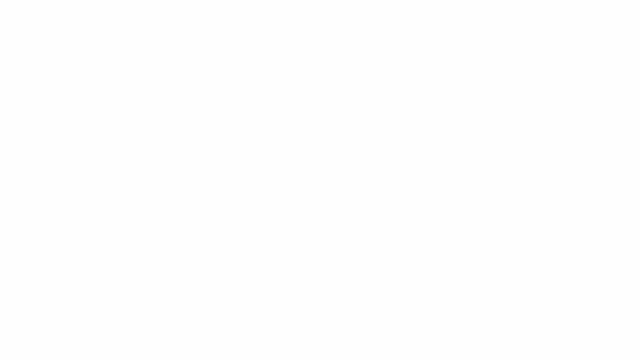 This is essentially what happens in radioactive decay. Isotopes that have unstable nuclei like this are known as radioactive isotopes or radioisotopes. In our hydrogen examples, tritium, are unstable and are hence radioisotopes of hydrogen. The more unstable a nucleus, the faster it will try to rearrange itself into a more stable. 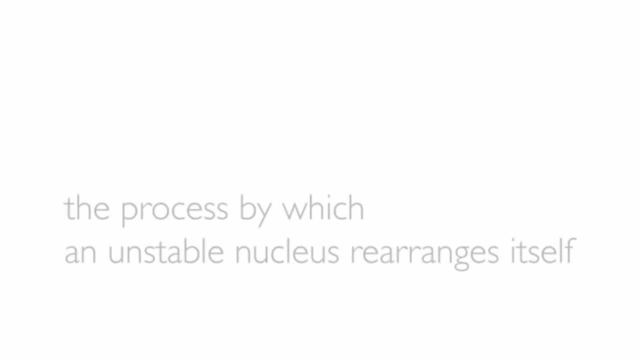 state, and another name for this process is radioactive decay. Radioisotopes are often used in medicine to trace aspects of body chemistry or blood flow. For example, a small amount of the radioisotope technetium-99 may be injected into the bloodstream. 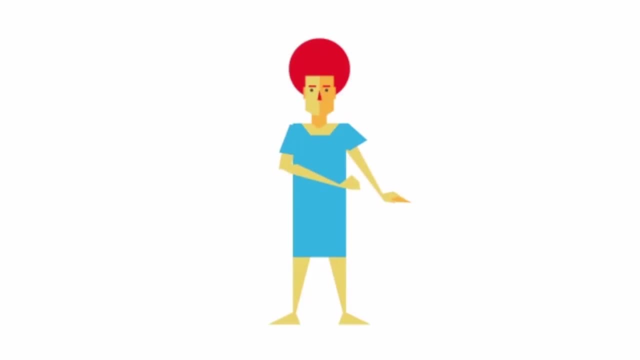 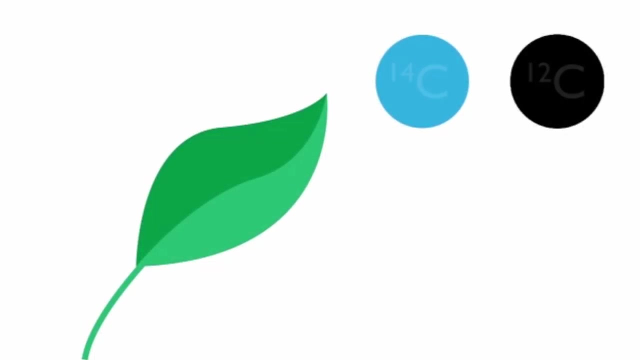 to show up on medical imaging and x-rays, And this is not a problem. It is known as a medical tracer. Tracers can be used by chemists to understand how a reaction works. Atoms of radioisotopes can act as markers, allowing chemists to follow how a reaction. 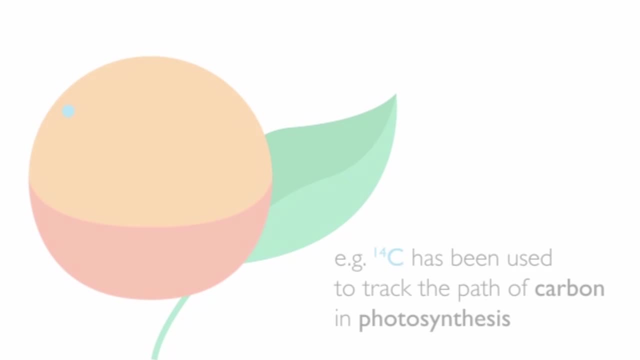 sequence occurs. And, of course, radioisotopes are also used in radiotherapy to kill malignant cancer cells. So, as you can see, isotopes are important in modern science, and so we'll finish with a summary of the key points. Isotopes of the same element have the same chemical properties.